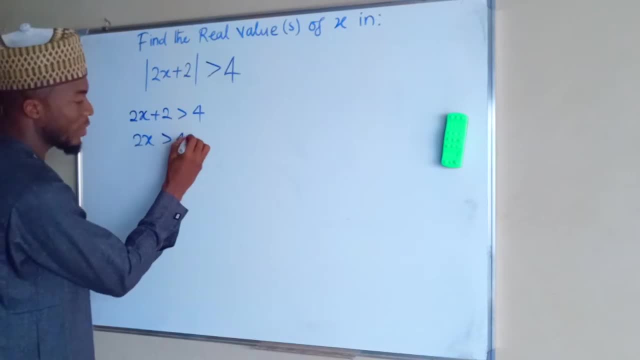 becomes negative 2. So we have 4 minus 2, and 2x now is greater than 2.. If you divide both sides by 2, you are going to obtain x greater than 1.. Then now we are going to assume that this value is negative. 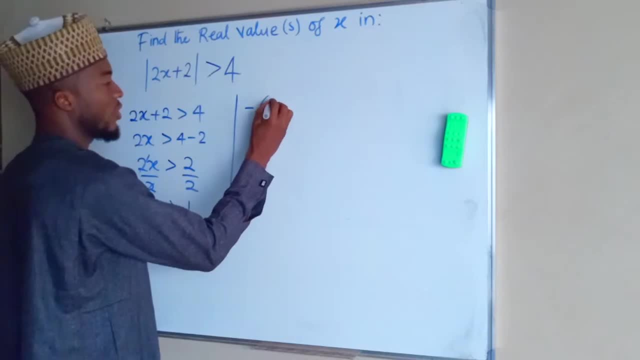 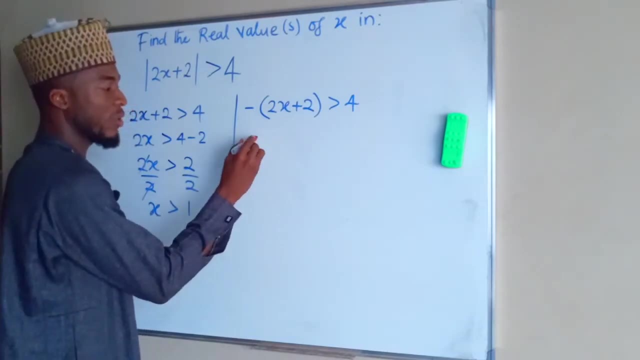 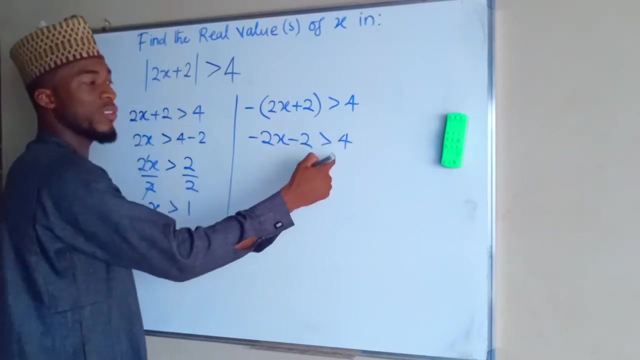 So for that case, we are going to have a negative of 2x plus 2 greater than 4.. If you expand this bracket, you are going to obtain minus 2x minus 2 greater than 4.. If minus 2 crosses the inequality sign, it becomes positive. so we have minus 2x greater than 4. 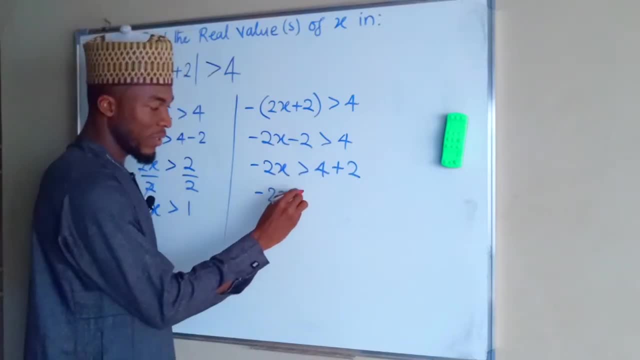 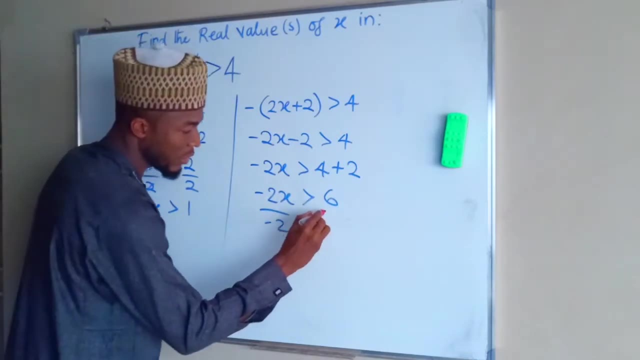 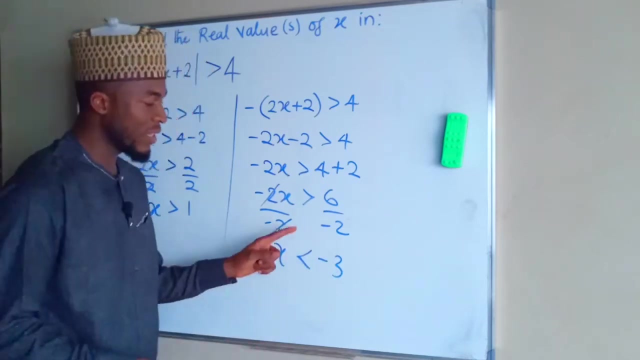 plus 2.. Minus 2x is greater than 4 plus 2, which is 6.. Now to solve for x, we divide both sides by a negative number: 2. This cancels this. then x is less than negative. 3. Here we have greater, or here we have less than. 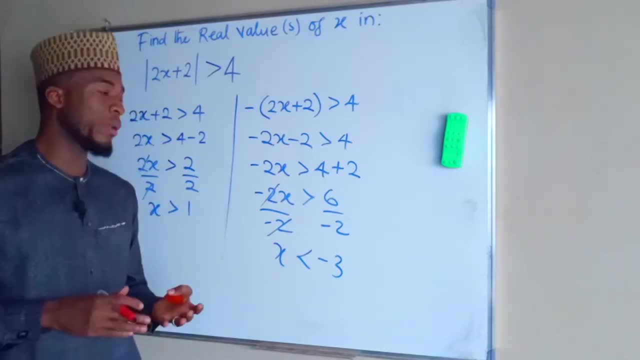 because the inequality says: if you divide or you multiply an inequality with a negative number, it changes the position of the inequality to a direction opposite. So we have now x greater than 1 and x less than negative 3. But the question we need to ask ourselves are these two values? 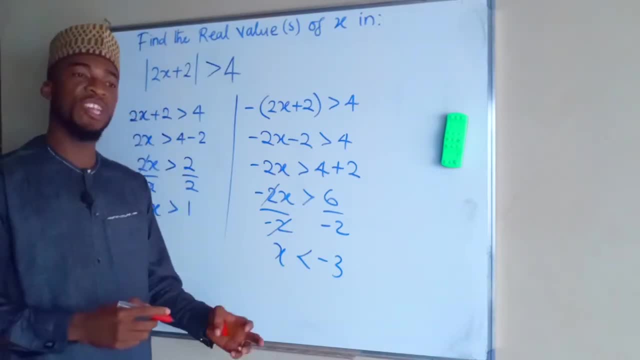 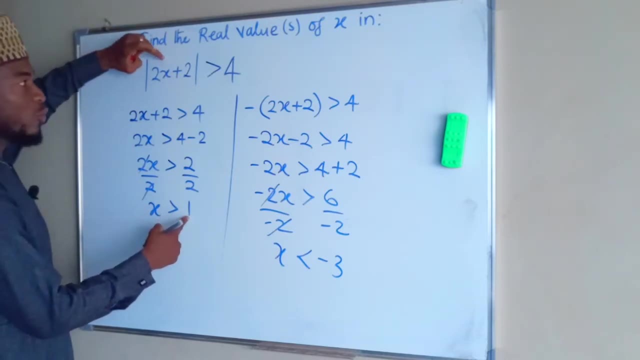 the real values of this x. For you to find out you need to check. So let's assume this x is positive. 1, then 1 times 2 is 2, then 2 plus 2 is going to give us 4.. The absolute value of 4 is 4, then is 4. 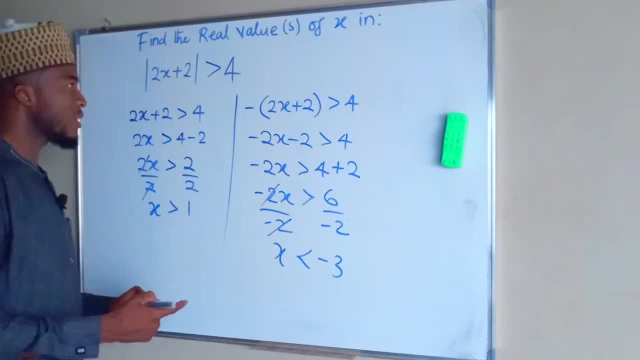 greater than 4?? Never, but equal to 4.. It is neither less than 4 nor greater than 4.. Therefore, this is 4.. Therefore, this is 4 greater than 4.. Never greater than 4.. Therefore, this is 4.. Therefore, this is 4.. 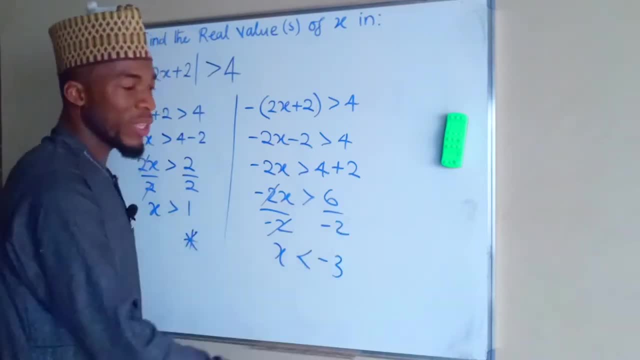 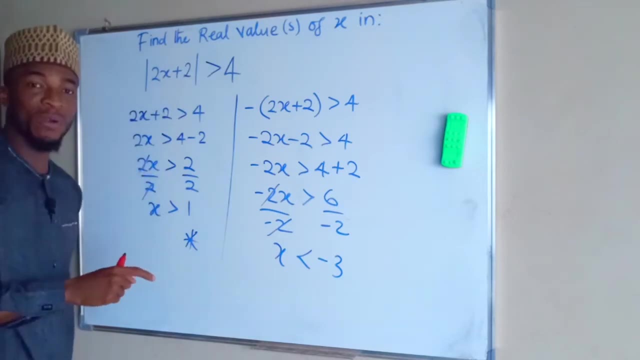 This is not a solution. Now we test for negative three. Negative three times two is negative six. Negative six plus two is negative four. Negative four in an absolute form is going to be positive And a positive four is never greater than four. 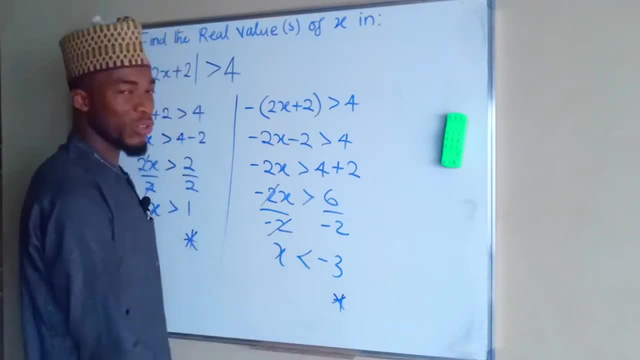 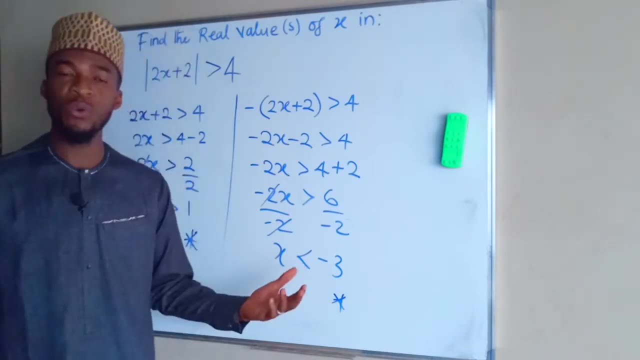 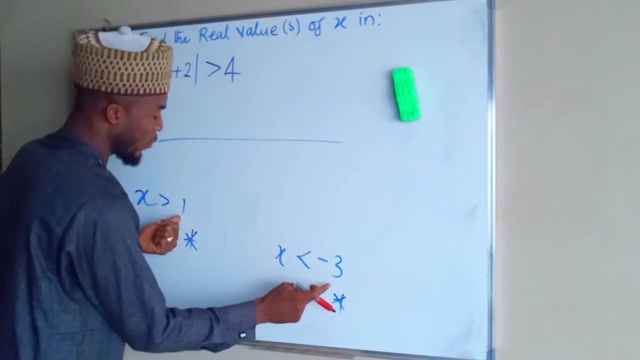 but equal to four. Therefore, this negative three is also not part of the solution. So how do we obtain the real solution? To obtain the real solution, we can do so on a number line. If this is a number line, we have positive one and negative three. 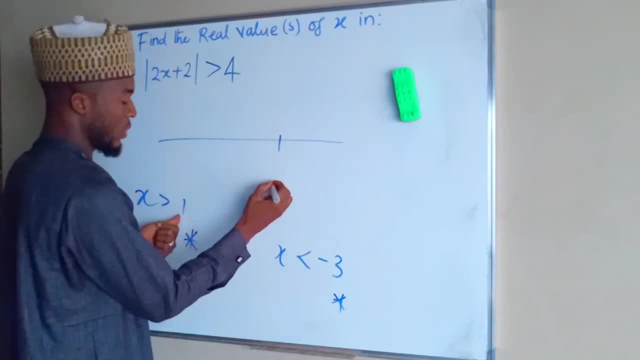 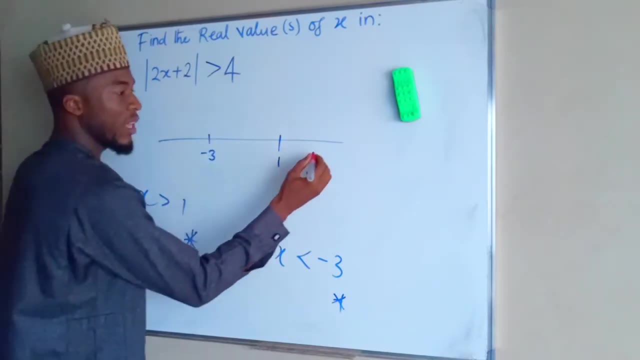 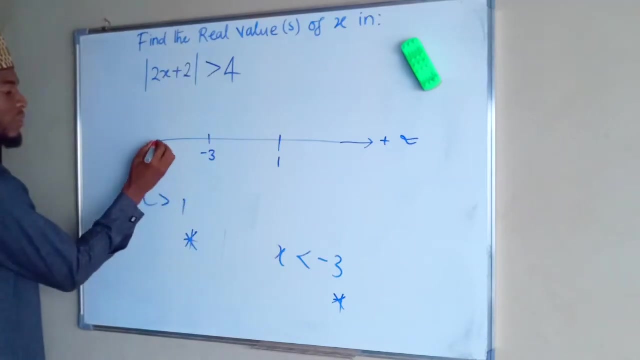 Positive one is greater than negative three. So we have positive one to the right-hand side And to the left-hand side. we have negative three. If you keep on going, you reach a certain number, which is a positive infinity- And to the left-hand side. 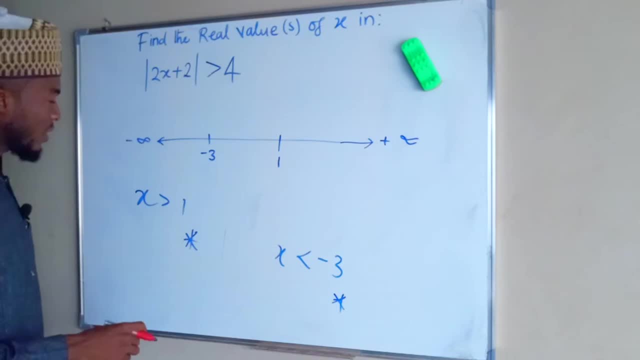 you are going to reach a certain number, which is a negative infinity. We have already tested positive one and negative three, and none of them satisfy this inequality, So we are going to cycle the two numbers. What we are going to do now is to test a number. 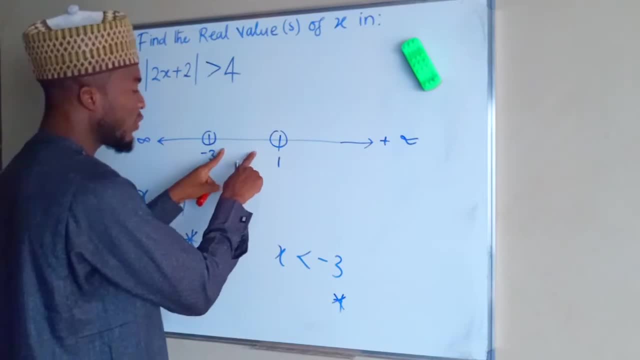 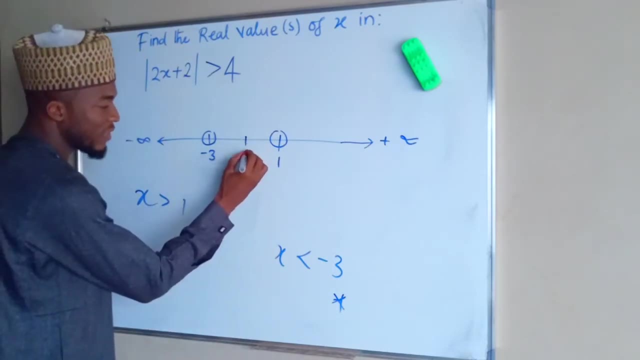 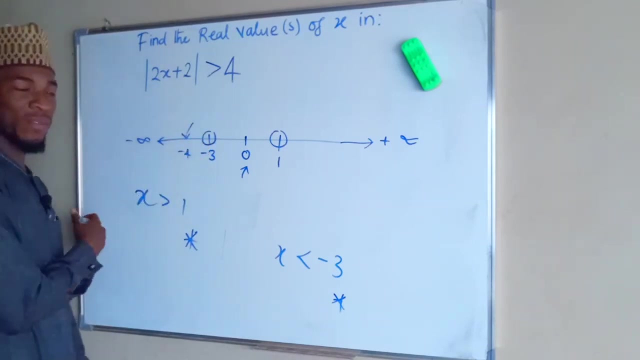 that is less than negative three, a number in between negative three and one and a number greater than positive one. We know that we can obtain zero here, so we test for zero. We can equally obtain a negative four here. We have negative five, and so on and so forth. 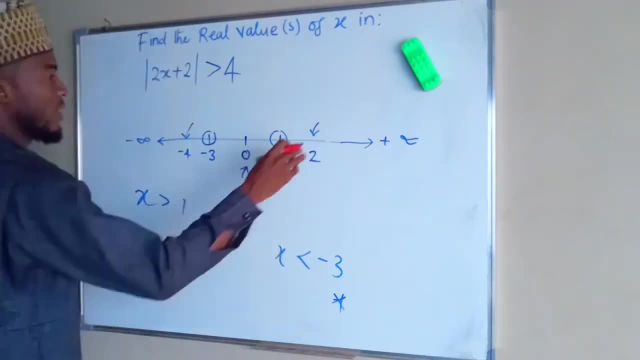 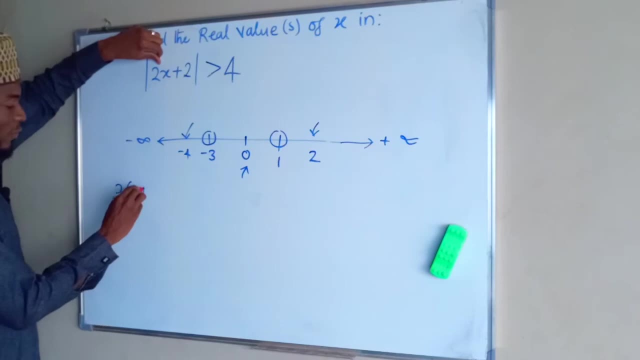 And we can get our number 2 or 3 here or 4.. If we take the value of x as negative 4, here we are going to obtain 2 multiplied by negative 4 plus 2. in an absolute form This time, this is negative 8 plus 2.. 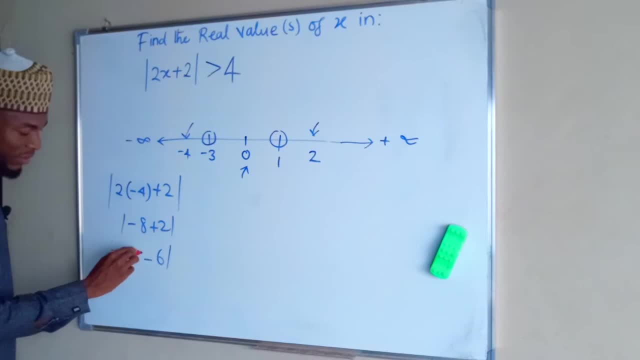 This will give us a negative 6.. In an absolute form, it will give us positive 6.. Then positive 6, is it greater than 4?? Yes, positive 6 is greater than 4.. Therefore, every other value within this range after a negative infinity will satisfy this inequality. 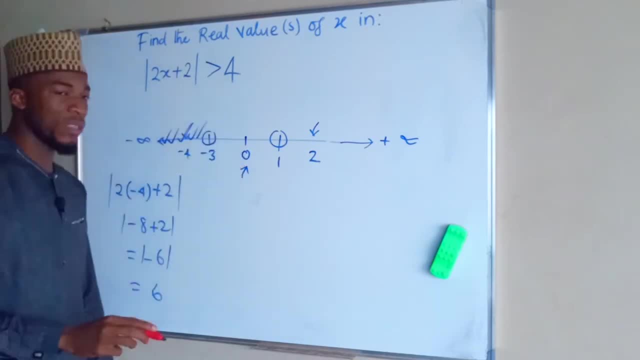 So all these values here will satisfy this inequality. Then, in between negative 3 and positive 1, we have 0, so we test it. We have 2 multiplied by 0 plus 2.. This will give us this time this is 0 plus 2.. 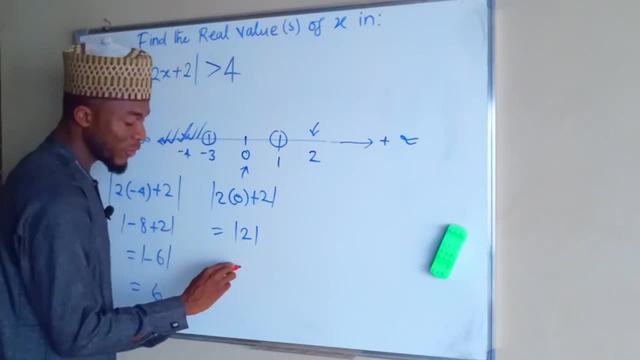 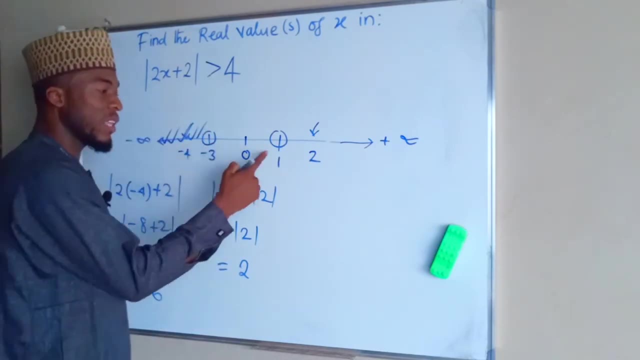 We have 2 in an absolute form and the 2 in absolute form is going to be 2 positive, And 2 positive is never greater than 4.. So therefore, between this negative 3 up to positive 1, none of the values there will satisfy this inequality.